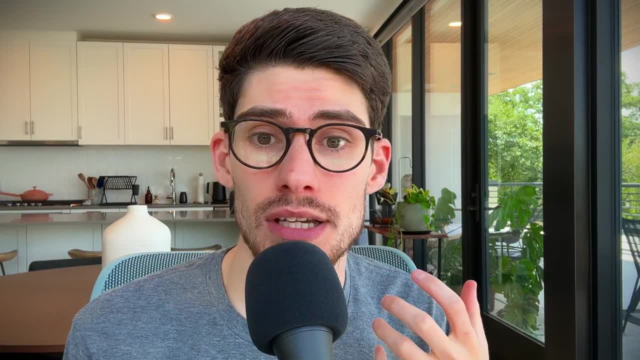 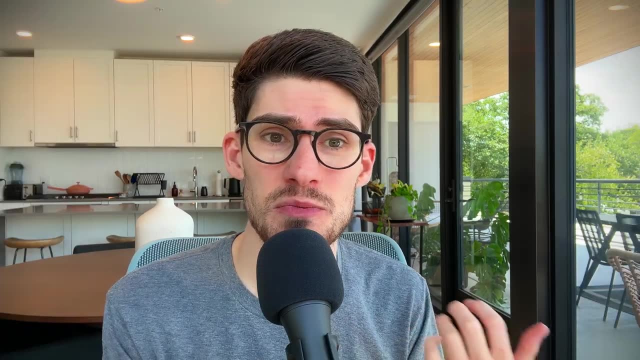 we used Shift for about a year. So I think the general concept that these tools are trying to do are so great, Like let's make the browser better, But I don't think that the browser is made better necessarily by just a Chrome extension, which is going to be limiting. 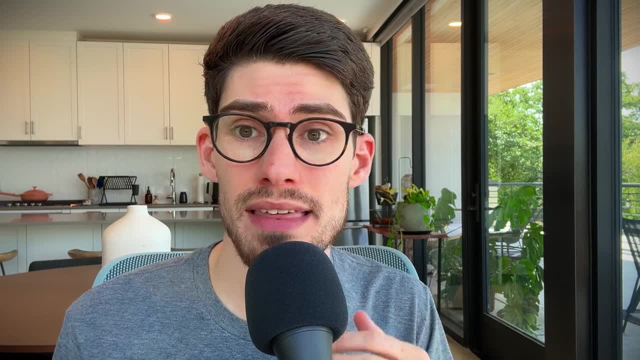 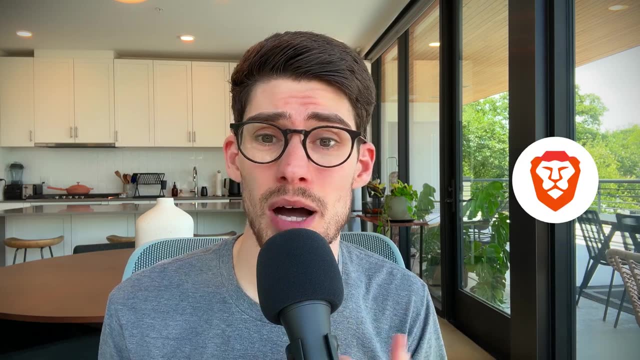 in so many facets. There's only so much that you can do to break that gap between Chrome extension and actual interface that you're working within. This is also the time where we started seeing tools like Brave, pop up and Vivaldi and heck, even Microsoft rebranding to Edge and being like 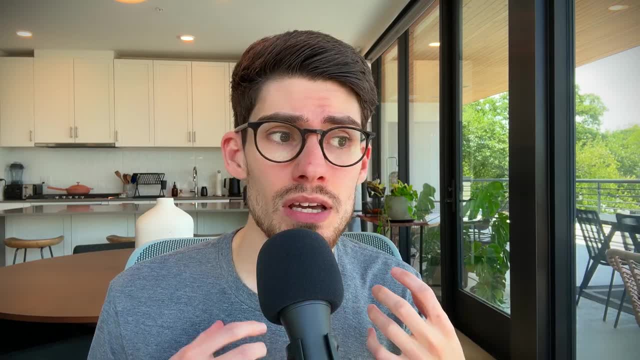 let's get back our Internet Explorer market share and introduce features in like open AI and things like that, And I think that's going to be something that we're going to see in the future. So I think that's going to be something that we're going to see in the future. 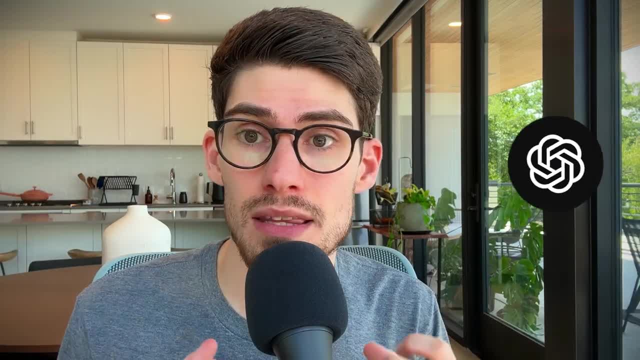 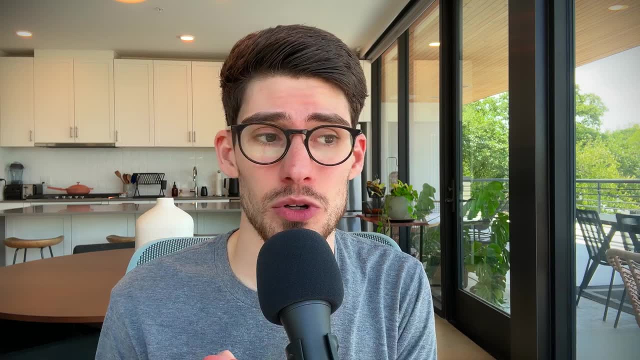 And GPT deep into the browser. They're trying to get the market share away from Google that they've taken. The problem is to have a good browser. you need it to work cross platform. You end up using the same languages that many of these other browsers are using to have them. 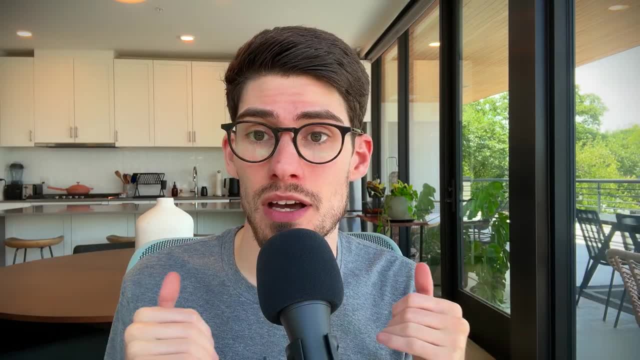 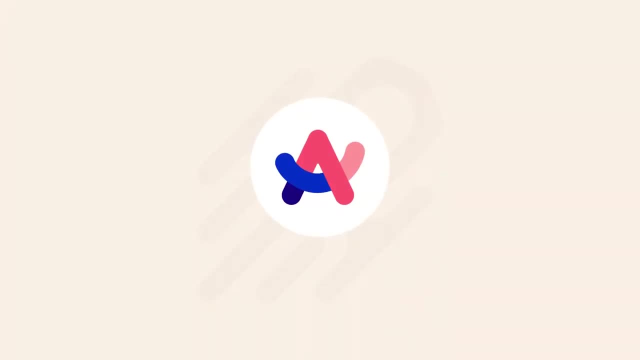 be cross platform. It almost stifles levels of innovation of just being able to build and iterate quickly. And that's where Arc has come out and totally changed the landscape, in that They are out of the gate, built atop of Chromium, but they're using Swift to build things out. So 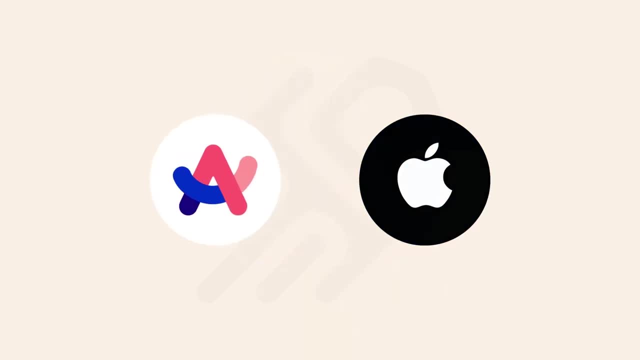 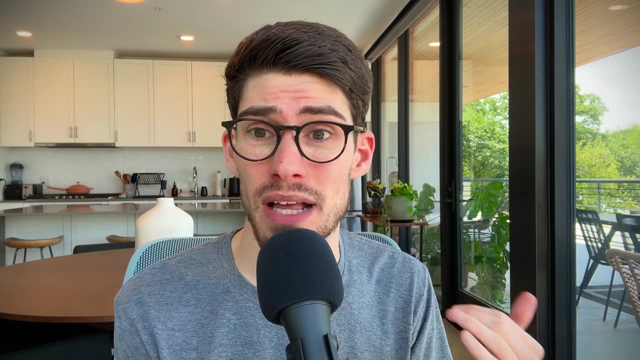 interactions and everything is just beautiful. The thing is it only works on Mac OS, And that is this risk, in a way that all these other browsers just wouldn't do out of the gate. They're like we need to be fully cross platform or we're dead. There's no way we're going to. 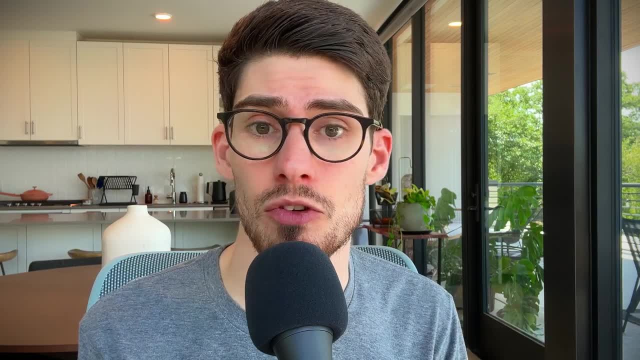 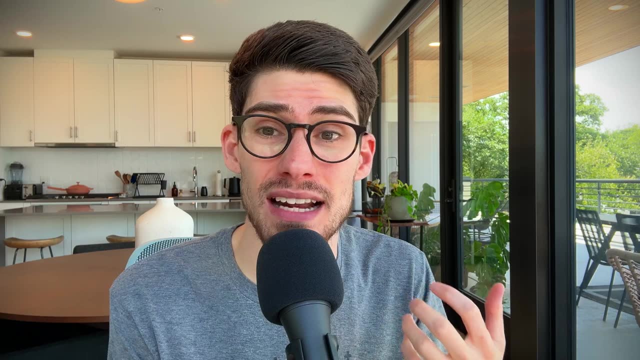 compete with Chrome and Safari if we can't do cross platform, And that's where Arc was like. well, hold on. What if we actually didn't care as much about cross platform out of the gate And we saw if we could actually innovate on this browser space that's been so stagnant? 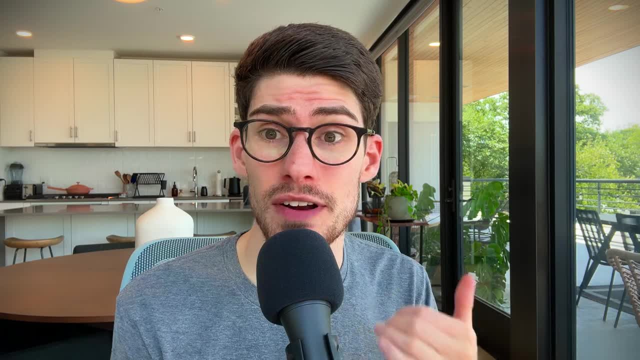 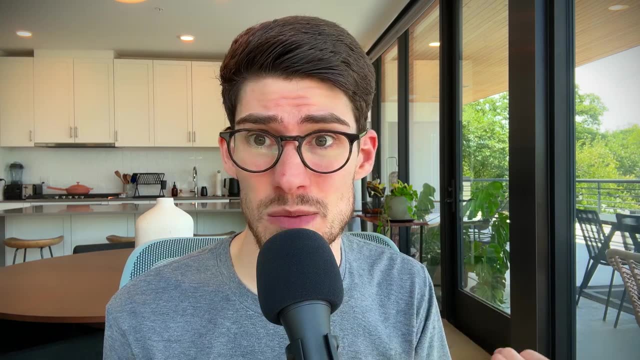 And that's exactly what they've done. By having a fresh foundation and a very specific customer base that they are focusing on- Mac OS users. that's enabled them to innovate and iterate so quickly in the space, which is actually the thing that is making them wildly successful. If you're currently 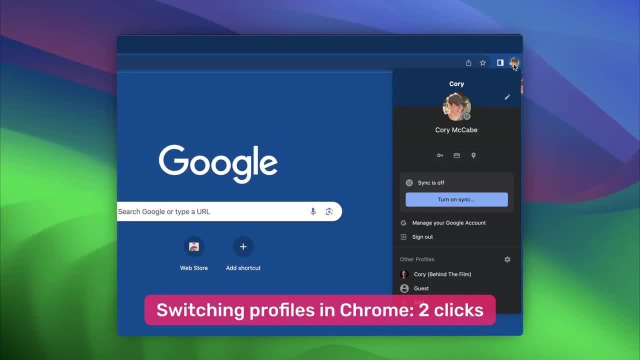 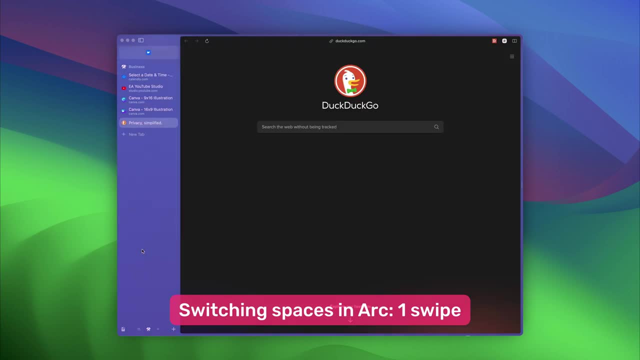 using a tool like Chrome. you're probably used to using profiles, which is like this hidden area that allows you to jump between, say, your work and personal. Well, Arc has this baked in at such a deep level that it is literally a swipe to the right and you're in a totally different space, or? 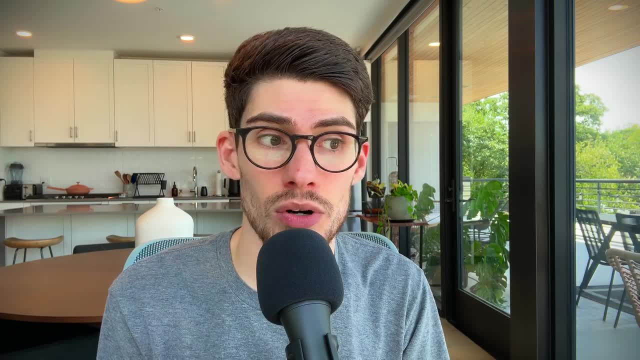 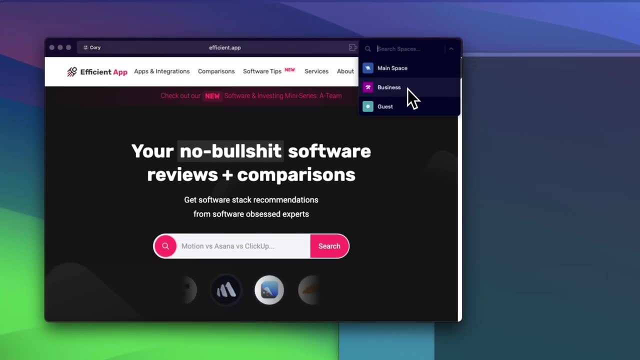 swipe to the left- totally different space. Or what if you're in Slack or Telegram or some chat messaging tool and you click on a link? it will pop up in the little Arc and you get to choose what environment you want to jump in. They have actually built these different profiles at such 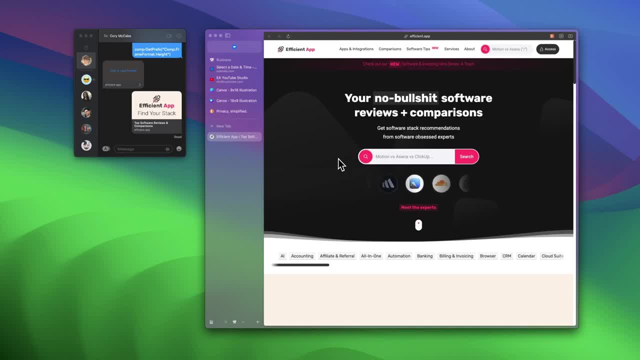 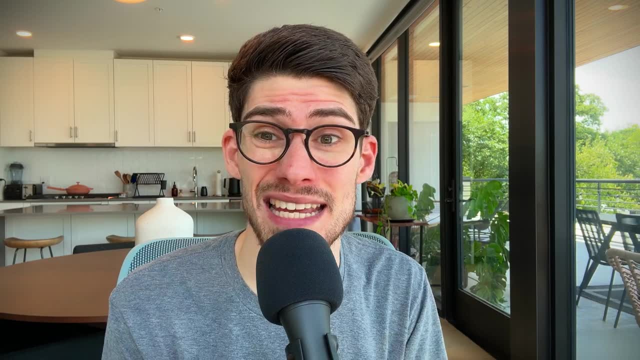 a deep level in the way that you're using it on a day-to-day basis With Arc. tabs are bookmarks and bookmarks are tabs. You're actually using the folder structure to access the pages that you're trying to use on a day-to-day basis. You're not just going through the folder structure to try. 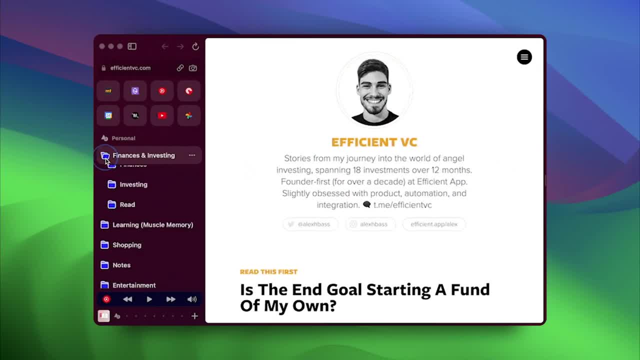 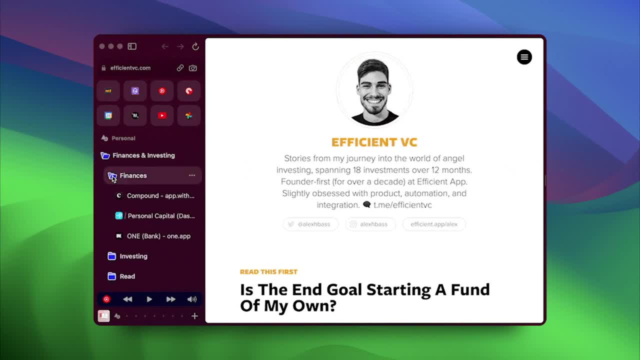 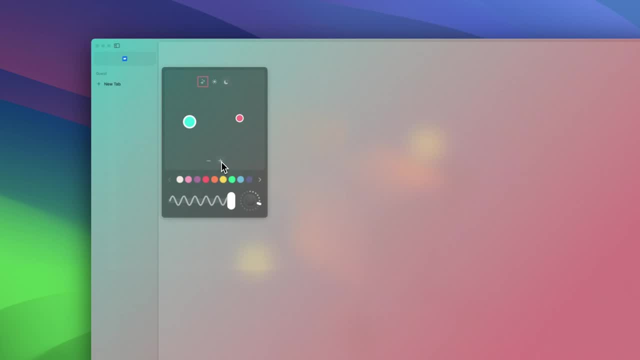 While it might sound weird at first, it is something that is impossible to move away from once you start using, And the truth of the matter is Arc is just fun to use. They let you choose all these different color themes and pin things, and it actually feels like you're using an. 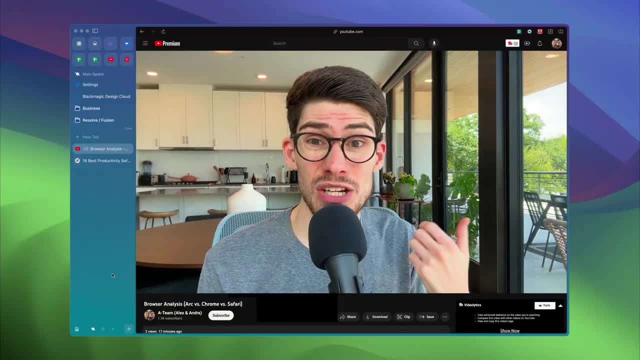 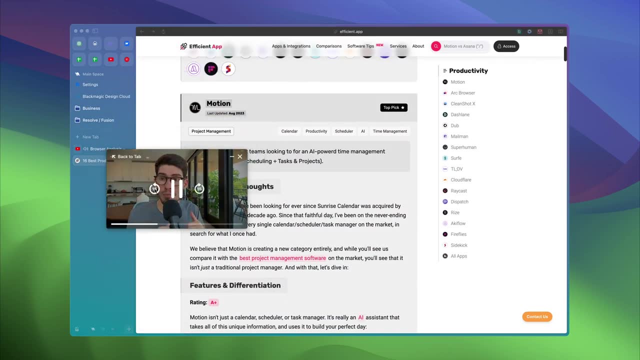 operating system, atop of what you're using. Play a YouTube video and then you leave the tab and then it pops out into a pop-up video that just works across your screen. These little tiny interactions that they implement at a deep level in just the day-to-day usage is really what makes it different. 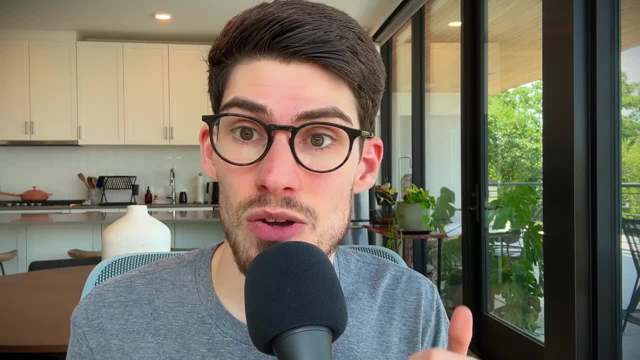 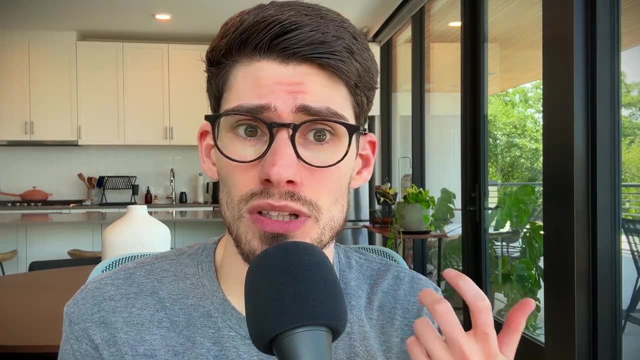 It is really the day-to-day experiences that you have when you're using it. For example, have you ever been on a website and you're trying to be focused in some of the work that you're doing, but then you click on a link and it brings you to a different website and a new tab, and then 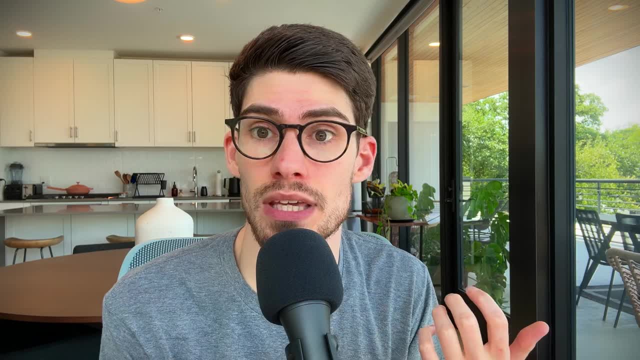 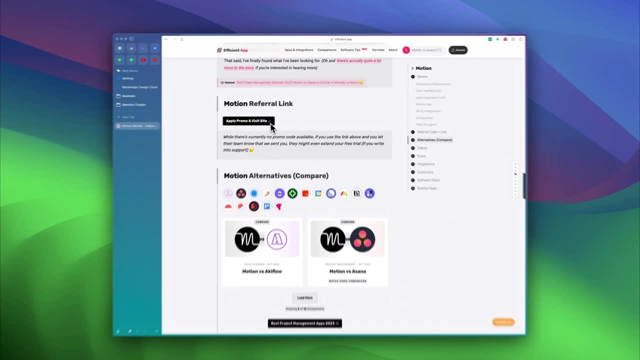 all of a sudden you go down this rabbit hole and then you're on YouTube. You don't even know what you're looking at anymore. With Arc they introduce such a simple feature called peak, where if you're on a website and you click an external link, it does a pop-up kind of interface where it's still 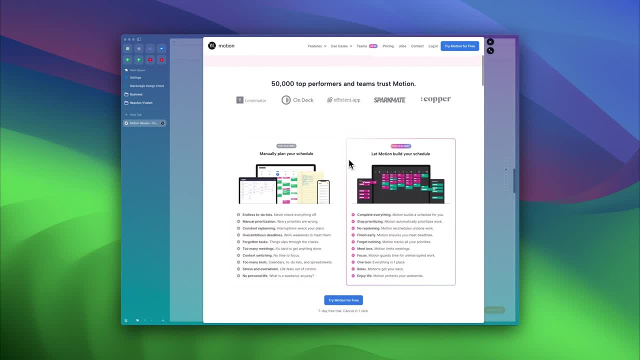 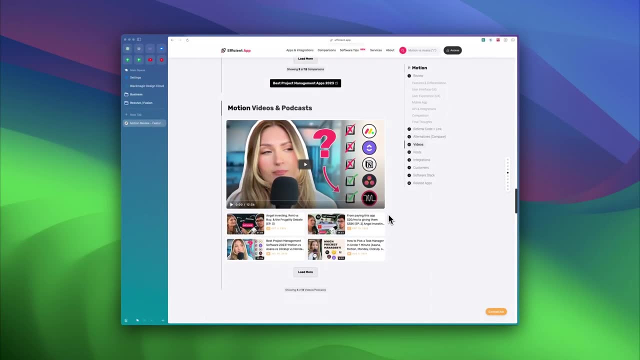 a layer atop of the tab that you're in. It's so clear where you were left off and you don't get as distracted because you're like, oh cool, I'm not going to leave this and go back to what I was doing. If you want to make it full screen, you can go and do that, but it's really an option that you 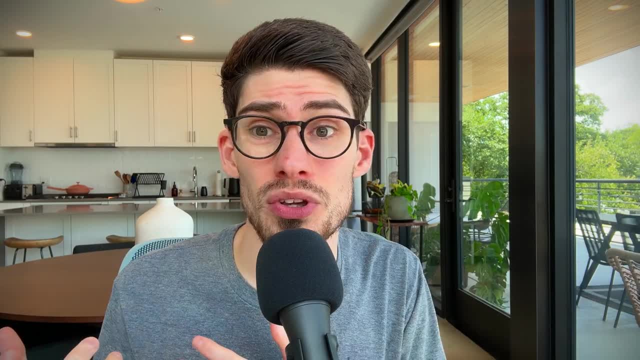 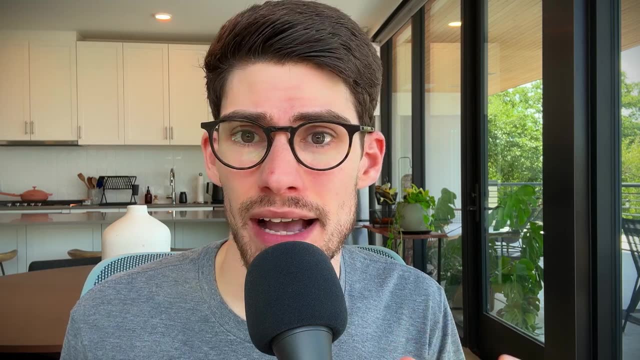 need to make the decision to do, versus it making that decision for you, which is most of the other browsers on the market right now. So, when it comes to actual productivity in your browser, it's more about those little interactions and what they're doing to help you be more productive, and 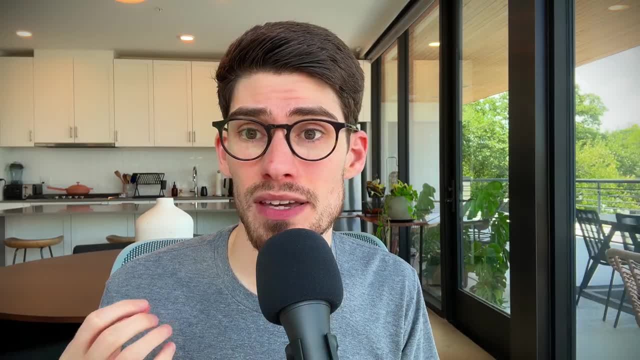 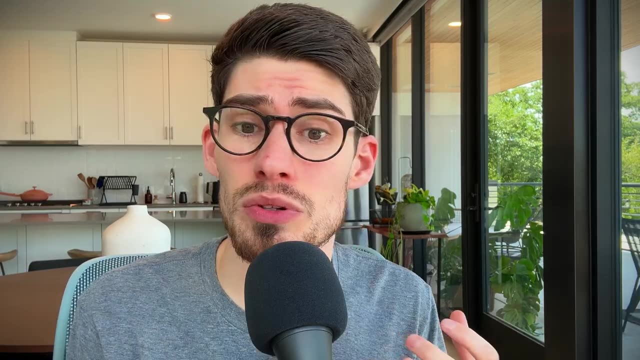 be aware when you're about to go down a time sink. It's not just about having your favorite apps pinned on the left-hand side that are quickly accessible. That doesn't make productivity, but that's the approach that tools like Sidekick Browser and 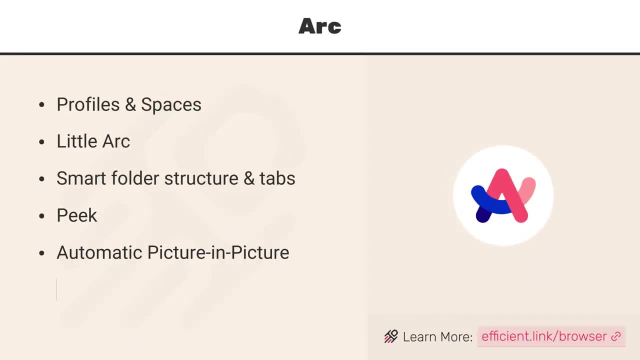 Shift are going in. That's not really productivity, though It's in the micro interactions and Arc has thought through them so deeply. Okay, let's switch to Chrome. You're likely using Chrome right now, as they own 60 plus percent of the browser market share. Love or hate Chrome, you have to appreciate. 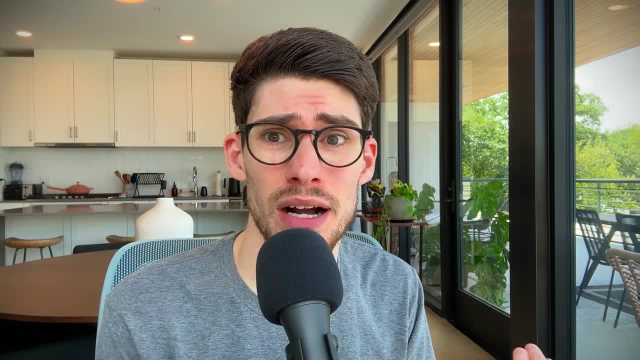 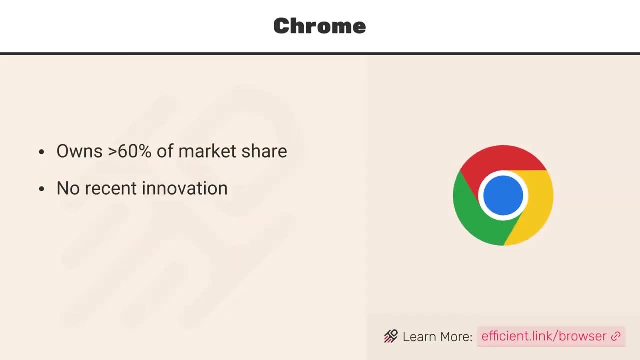 it. Without Chrome, Chromium wouldn't exist, and then your favorite browser also probably wouldn't exist. Chrome innovated a lot early on, but then, as the deep ties to Google existed with search, they really couldn't build the level of productivity into it, because that actually 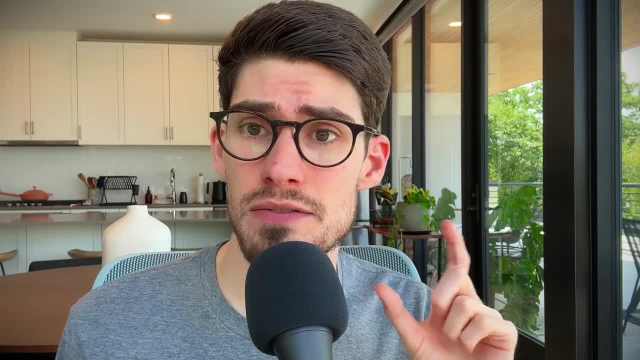 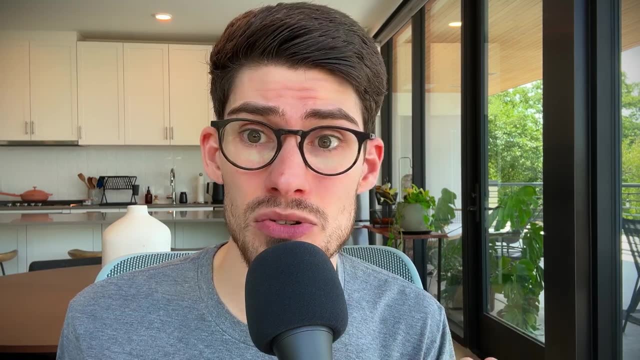 hurts their ad revenue business for actually searching Google. There's this very weird alignment that also causes inertia to happen, where people are just used to doing what they're doing. They're used to opening up that new tab and searching Google to literally find what they. 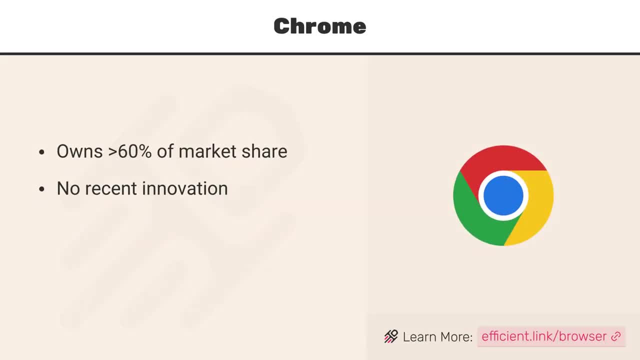 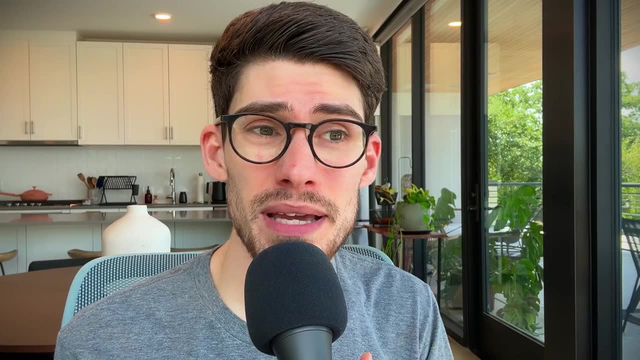 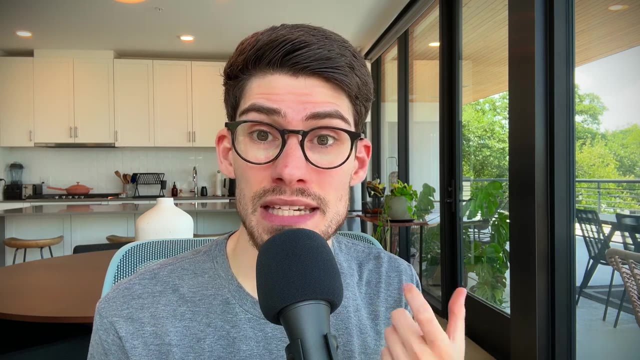 already had bookmarked the week prior, And Google likes that, because now you're more ad revenue for Google On the plus side. Chrome just works. Businesses use it. They have billions of users. The biggest problem that comes with that, though, is they can't make major changes. Imagine making a change that affects billions of daily 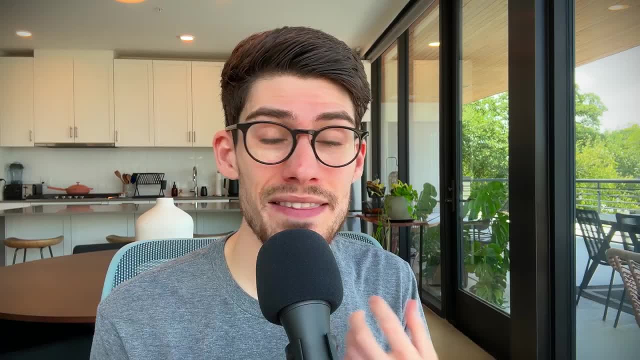 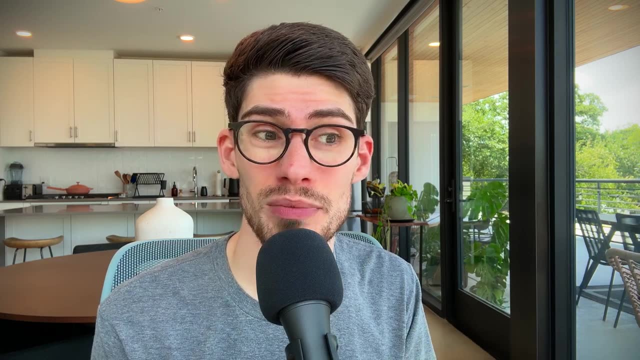 active users. You're going to upset a lot of people, and this is where the inertia comes in at play. at such a deep level, People don't want change, and those are the people that are using Chrome, and Chrome does what it needs to do and it does it well, But it looks pretty much the 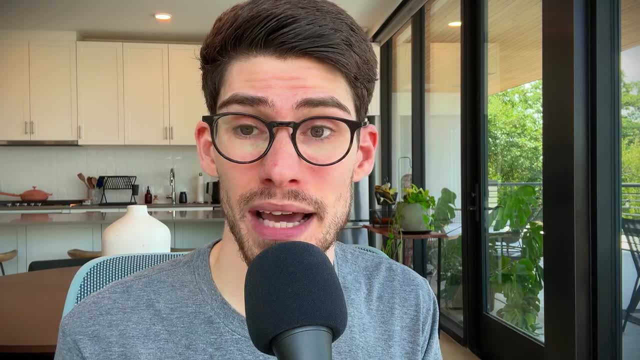 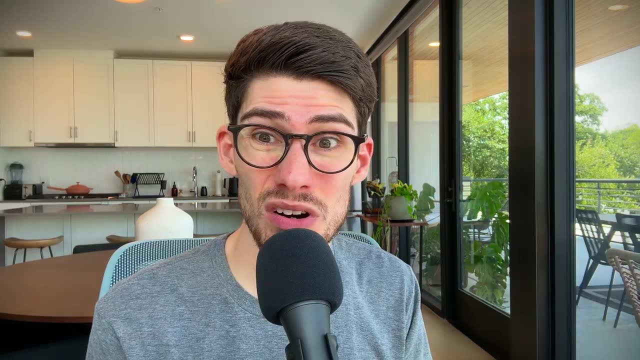 same as it looks six years ago and it's going to look the same six years from now. That's Chrome. It's stable. Businesses can rely on it. They're not going to have these major issues. The main thing is they just need to work and it needs to be stable. That's Chrome, So let's switch gears to. 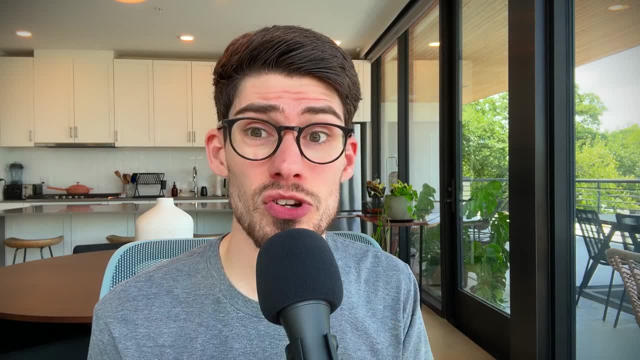 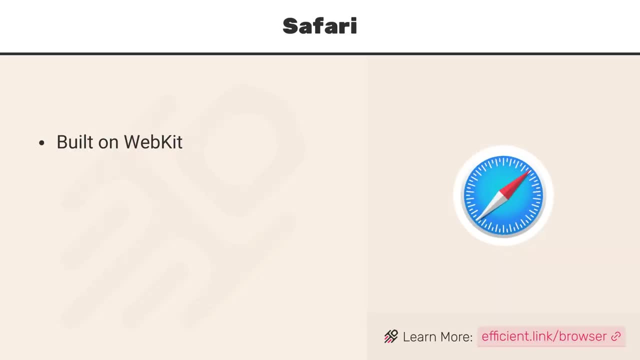 Safari. The interesting thing about Safari is that Apple chose very specifically not to build it on Chromium. They wanted to go their own path using WebKit because they, kind of like Google, wanted to own the foundation of the way that people access the internet. Safari has focused a lot on trying. 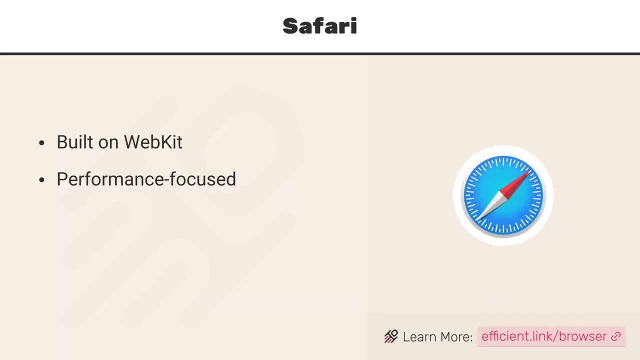 to just be a performant browser that doesn't burn too much battery life, And it's just a really good companion to Mac OS and iPhone. Yeah, So the big negatives here is it just doesn't work on other devices, So you can't use it on Android, You can't use it on 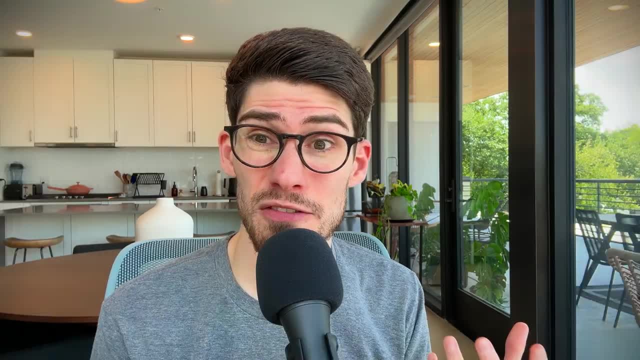 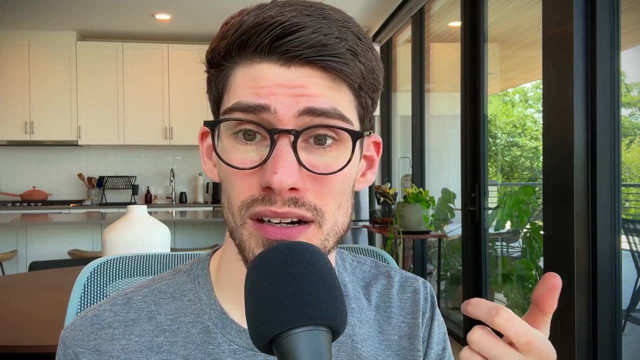 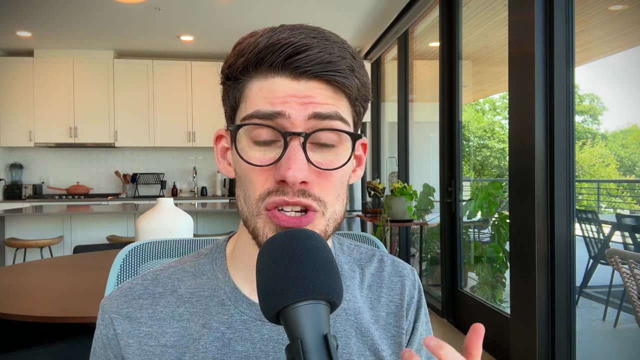 Windows. They really want you in their ecosystem to use it. by focusing specifically on Mac OS, They really have been able to tie that hardware in with the software, And that is a pretty big benefit. with that, though, They are making these decisions to tie in Safari like deeply to your. 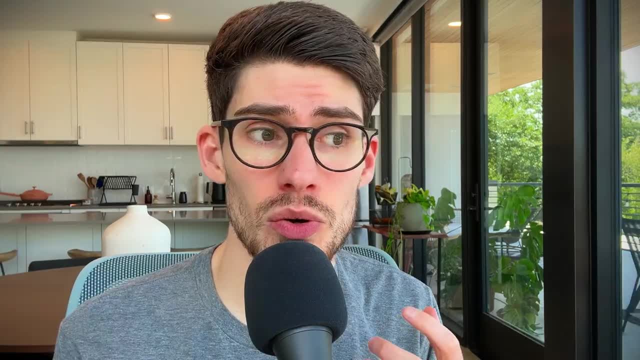 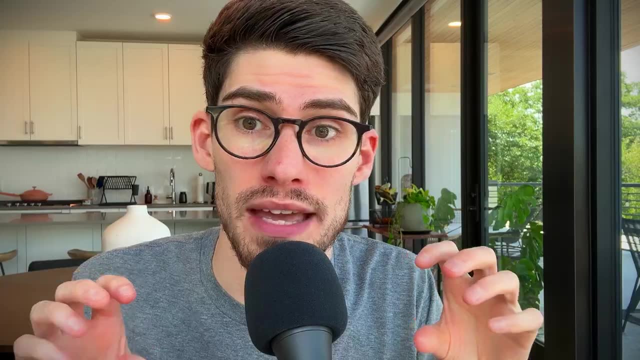 iCloud And, of course, Apple wants you to be able to use it for a lot of different things. So you pay for iCloud, So they want you on their infrastructure and their system. Everyone's kind of vying for your information and for you to get lock ins into what they have. So, while they may, 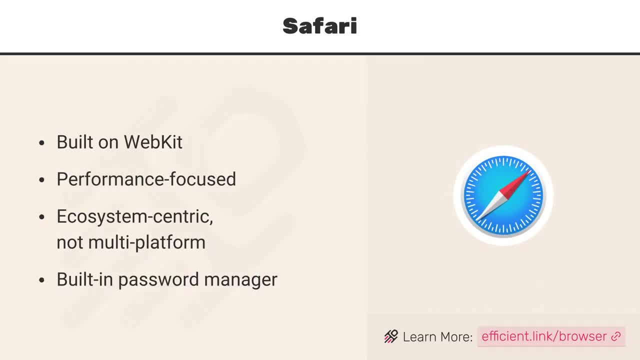 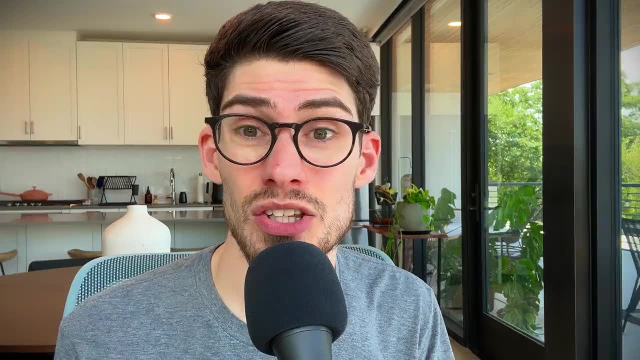 be introducing pretty cool features like a baked in password manager that allows you to unlock and log in to pretty much any website with your fingerprint. that's awesome, But it's not universal. You literally have to always be using Apple Safari and Apple devices to be able to. 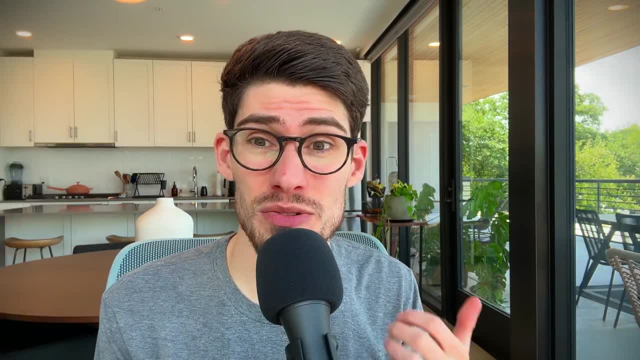 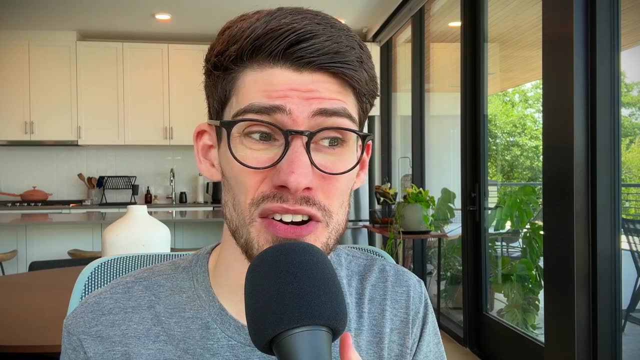 access this. This is actually something that our video producer, Corey, who's editing this video, could probably chime in better than me about, because he just switched to Arc from Safari after using Safari religiously for years. If anyone knows me, I try to convince people to use Arc when 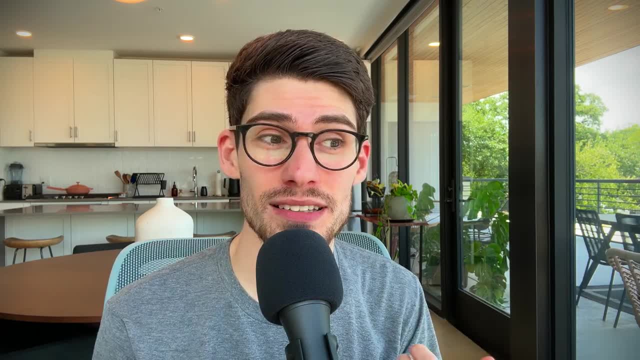 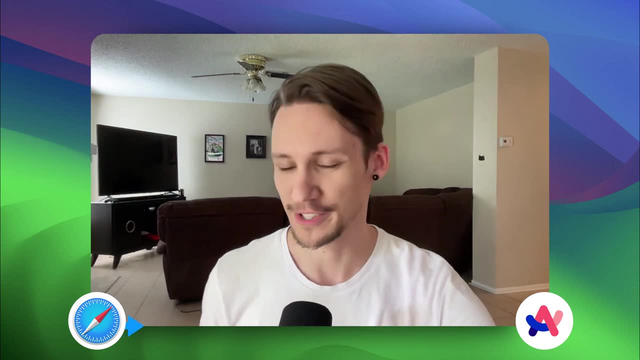 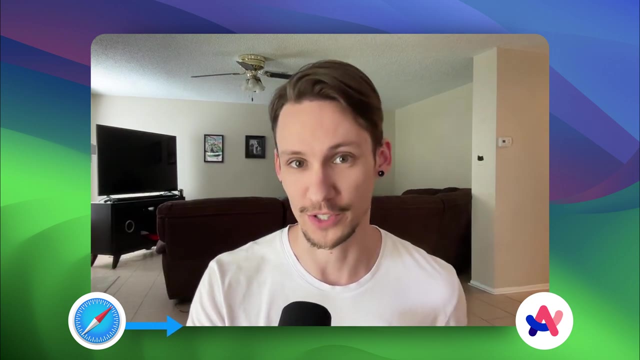 I first start meeting them. So that was no different with Corey, And there were hours of debates going on every time we hung out. Corey McLaughlin- Hey, I'm Corey- And yeah, like Alex mentioned, we had hours of conversations about Arc and Safari. My story is that I didn't have a pain point or a problem to solve. I 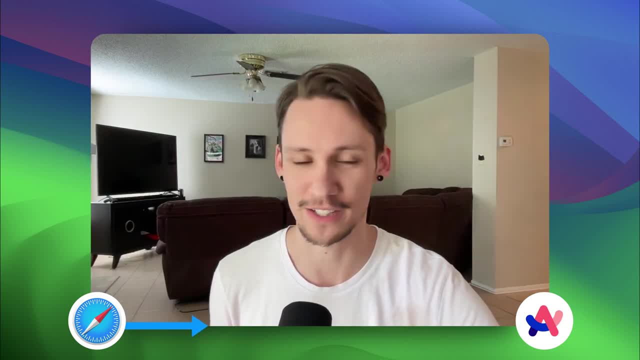 happy with Safari. It's more efficient on my computer, CPU wise, than Chrome, because I used to use Chrome, Even though I didn't have a pain point. just finding out that Alex literally bought a MacBook just to use Arc was like OK, this guy's pretty serious about this browser, So I had to. 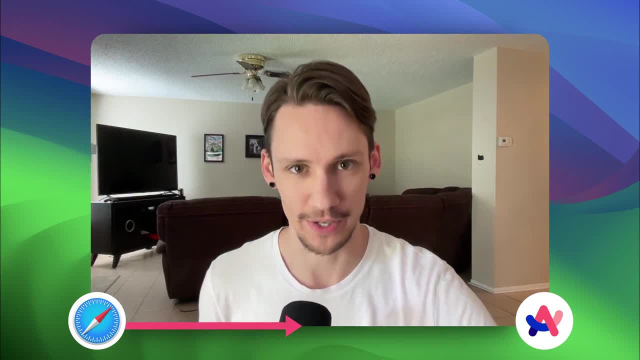 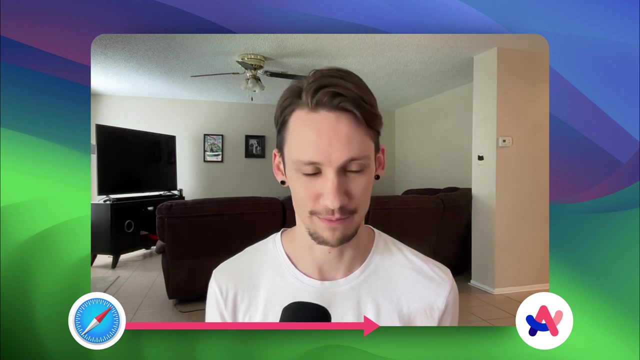 give it a try And I couldn't deny the unique experience and also just how fun and like it had its own like energetic nature to it that I just really enjoyed when I was using it. But I actually went back to Safari after trying Arc for the first time because I missed my like passwords and 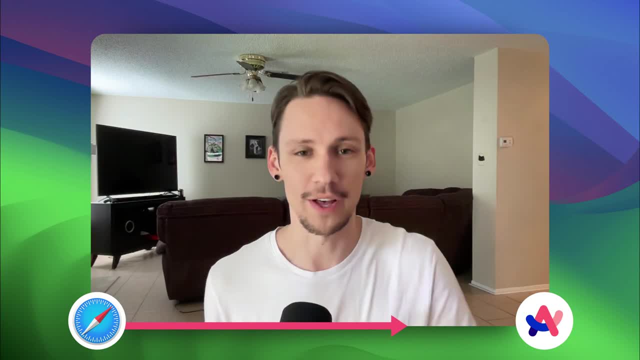 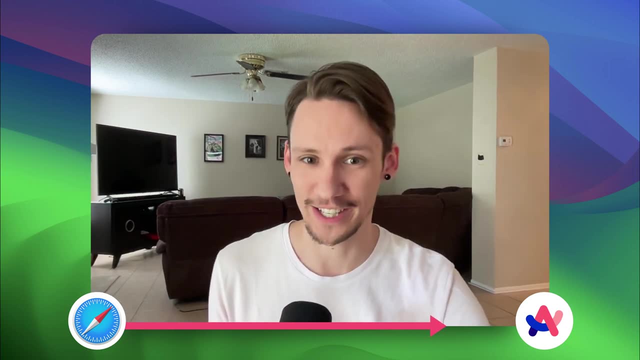 like Apple Pay and things autofill, all those things. But there are solutions to fix that. So I tried Arc for a second time. So I kind of went back and forth a little bit, And after trying Arc a second time I haven't moved back since. I've been pretty much fully on Arc now, Like I might. 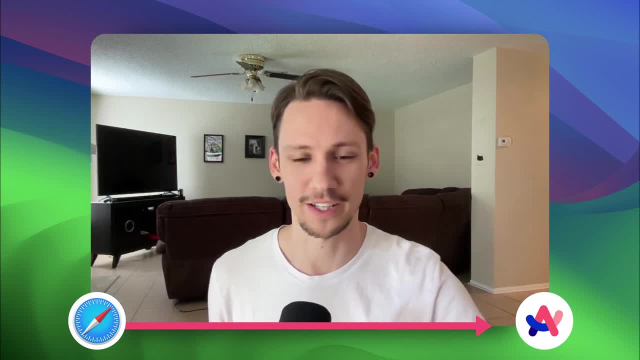 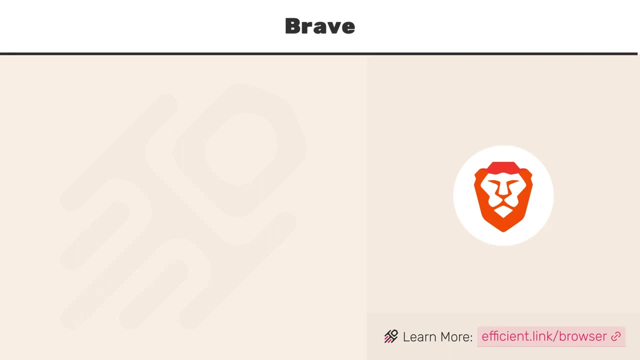 have like two percent of things that I use Safari for still, but like, slowly and slowly that's getting to 100 percent fully using Arc now And I love it. If you've heard of Brave, you're probably a privacy focused individual, someone that doesn't. 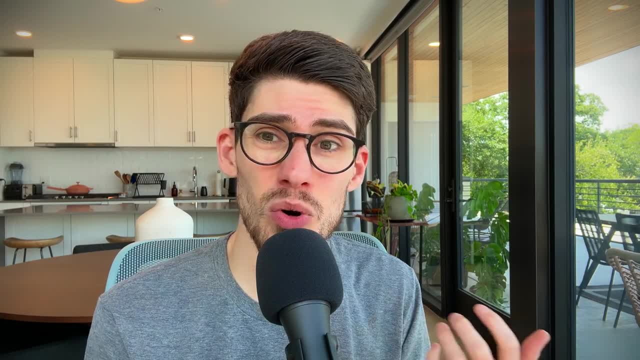 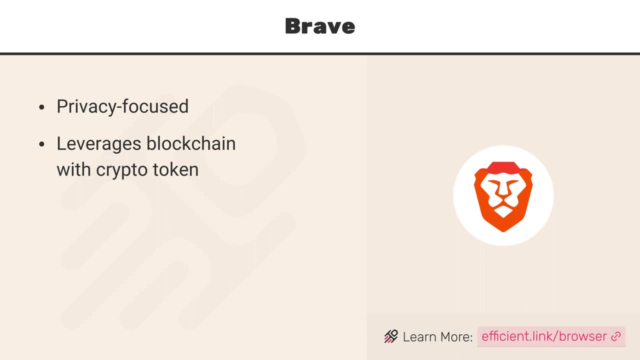 want Google to own all of your information and is typically more geared toward the blockchain and crypto in general. That was where they first started building out, and they had a crypto token tied, So you would actually get compensated by visiting websites, And in a way, it was like. 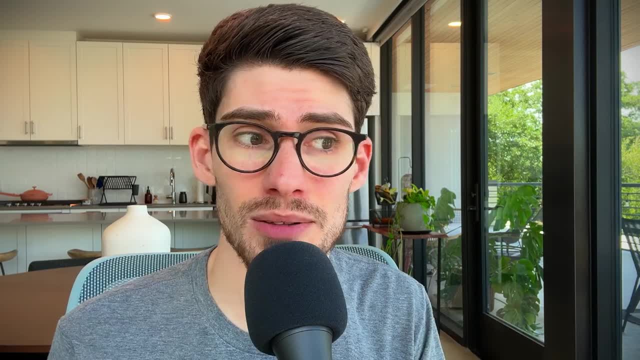 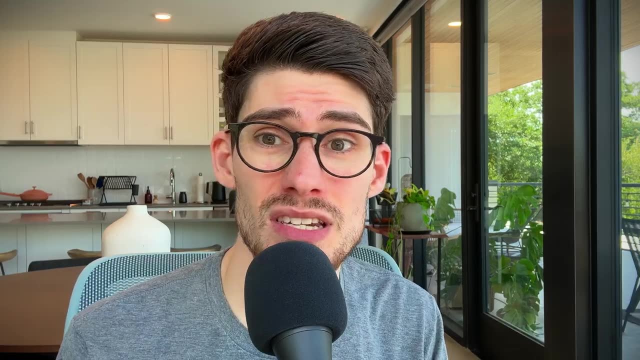 you should own your data and you should even be compensated for your data. It was a really cool idea. It's built on Chromium, So it's the same type of foundation as Arc and Chrome, But the main gist of it is it's privacy focused, So you don't have to give them an email. 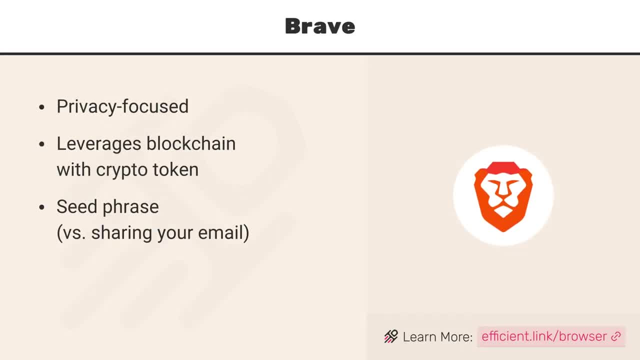 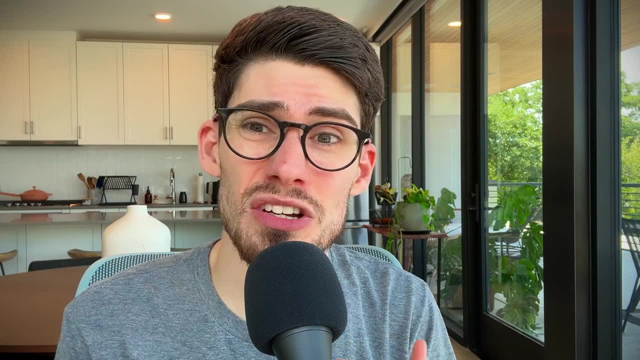 You could essentially just use a seed phrase And that's what all of your bookmarks and everything are backed up to, And people that are super privacy minded they really appreciate that. But that's also not going to give you as good of an experience as having an actual account tied. 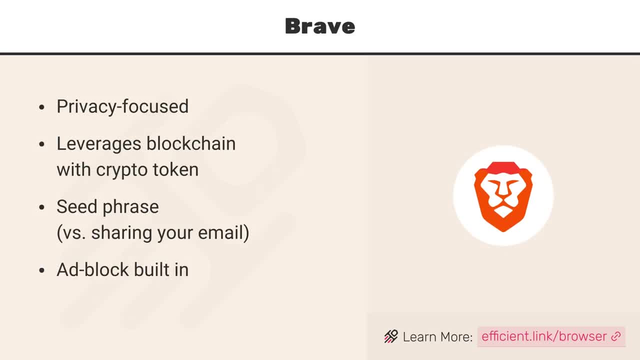 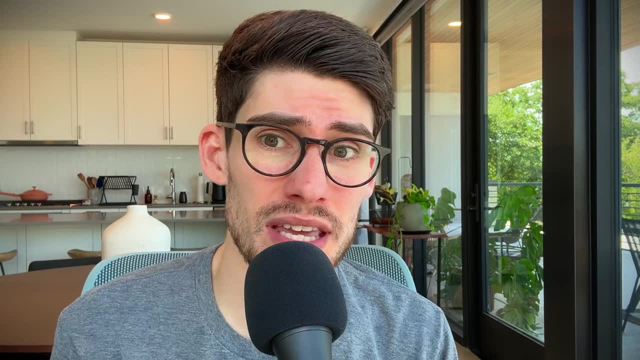 to what you're doing. Brave has things like Adblock baked in quite deeply at the foundation. They also support Chromium extensions, like everything else that you're used to. It's really impressive with what they've done, but that's also going to help you get more. 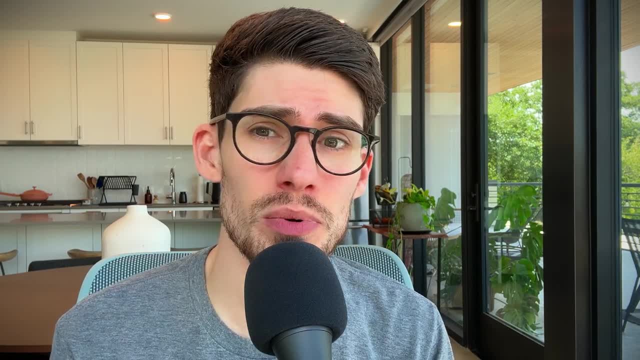 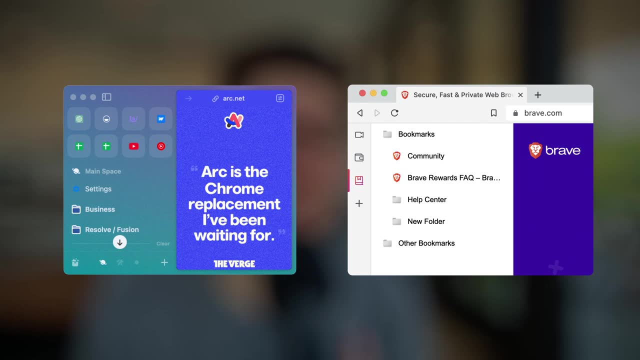 experience, And I think that's going to bring with it many limitations as you actually start getting into super innovative features. On top of that, they've also taken a little bit of inspiration from Arc in the way that they recently rolled out a sidebar navigation. 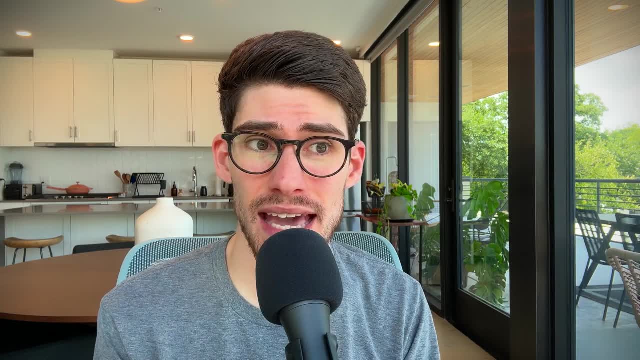 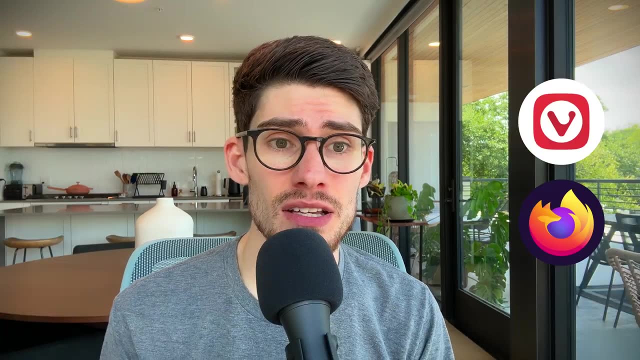 I think all that really shows is Arc is onto something and their biggest competitors are taking inspiration. Okay, now I just want to go through like Vivaldi and Firefox. So Firefox, for example, that was like the leader in the space, And there's so much. 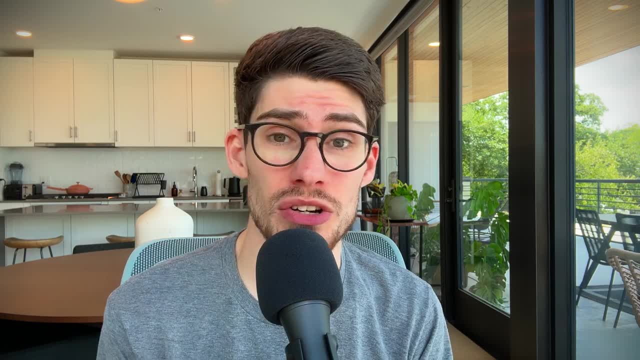 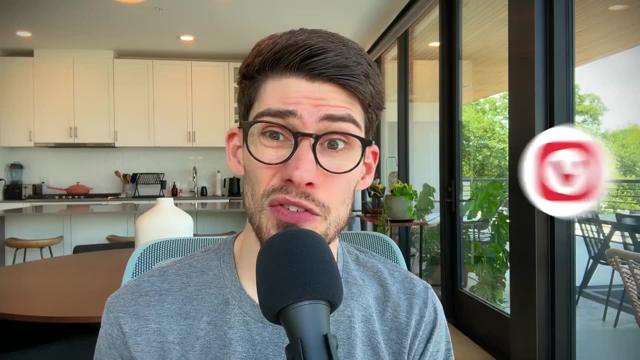 coming out. That was my main browser for many years, before even switching to Chrome, And they were innovating a lot back then, But now it all just kind of feels much of the same. Even Vivaldi, they started moving more into the personalization and you can do color themes and 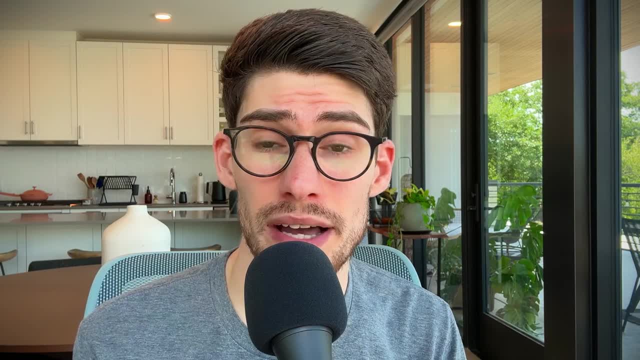 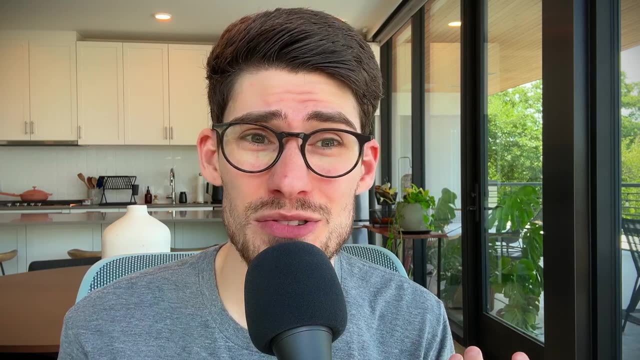 really get kind of fun with that, And they had the sidebar tab navigation as well, But I think they've all kind of struggled to really be anything super special. The craziest part to all of this is most of these browsers business models are. let's make our money by getting Google to pay.